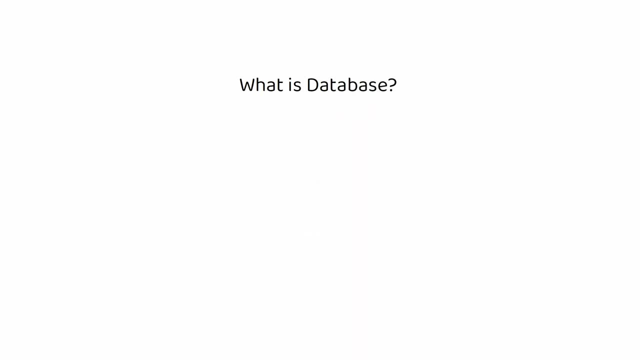 purpose of storing them. What is database? Database can be considered as a container filled with data or information which is electronically stored. For example, you can store a piece of paper, a piece of stored in a computer system. data in any form can be stored into the database. the 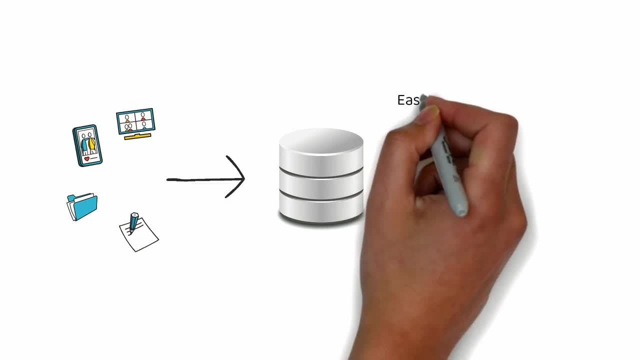 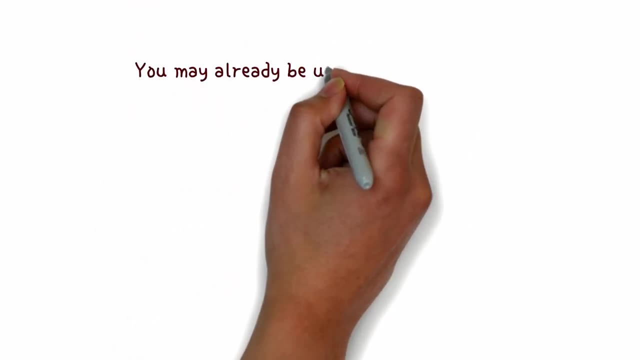 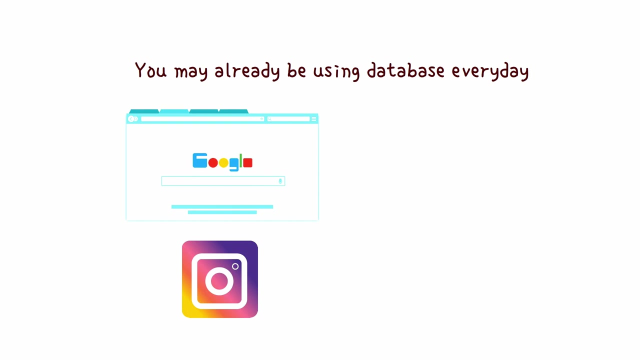 purpose of storing the data into the database is so it can be easily accessed, modified, protected and analyzed. you may already be using database in your day-to-day activities, because most of the websites or mobile applications today, such as Google, Instagram, whatsapp, Facebook, already use database to store. 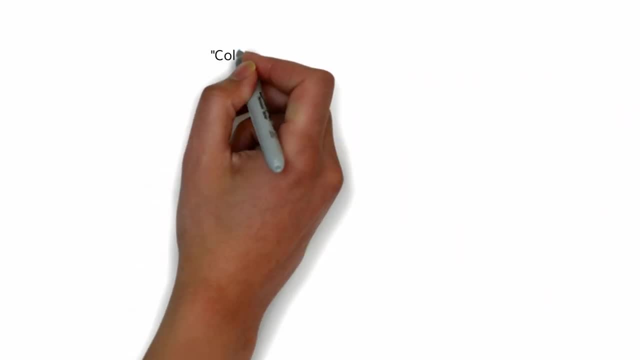 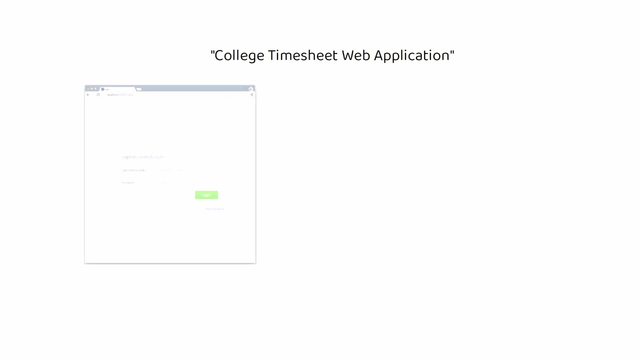 data. as an example, let's say, for your college demo project, you plan to develop a simple college timesheet web application. basically, this application should allow you to login through a URL and then have options to enter staff details, timesheet details, student attendants, student marks, etc. since this, 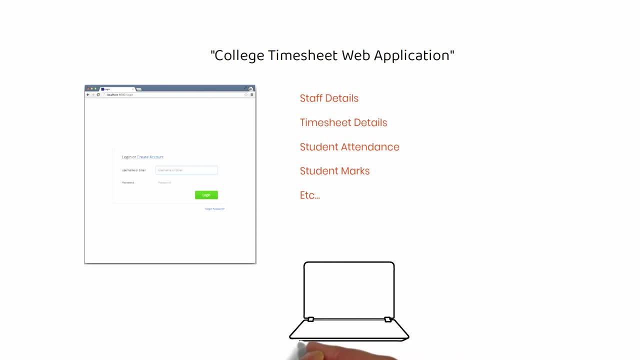 is a college demo project. you may just use your personal computer to develop this project. the first thing your application will need is your computer data storage file. open your computer and turn off and tick the logout and support your application. THANK YOU database. to store and retrieve the data, Hence you need to first install a 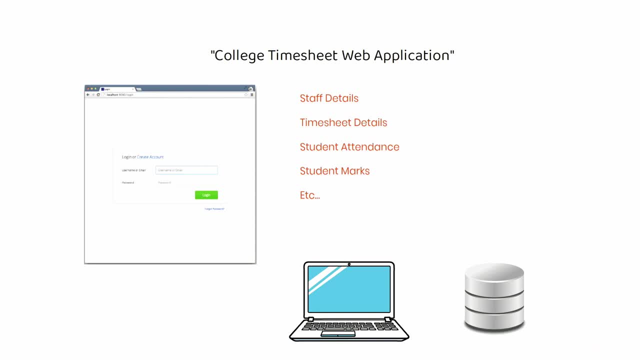 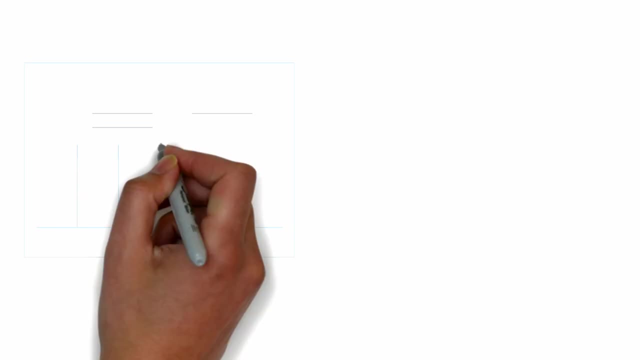 database on your laptop, which will connect to this timesheet application. Like any other software installed on your computer, database software will also be allocated to a specific location in your computer hard drive Through your web application whenever you try to save, edit or retrieve information. the 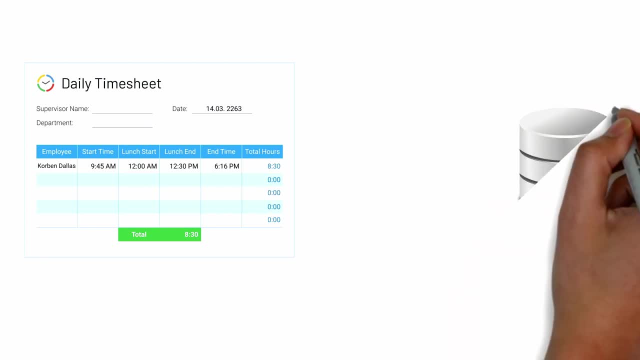 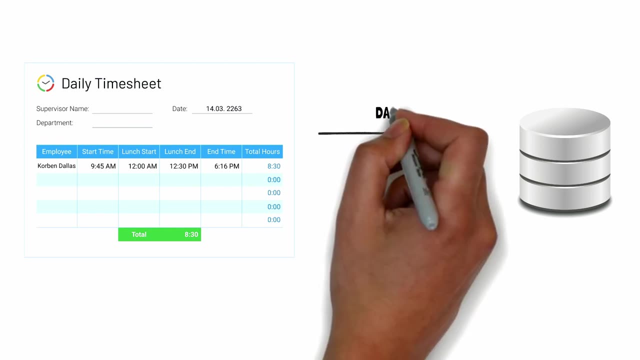 application will actually connect to the database to store, modify or extract the data. In other words, any information that is shown in your application is actually being retrieved from the database and any information you enter in the application will actually be stored into the database. But since the 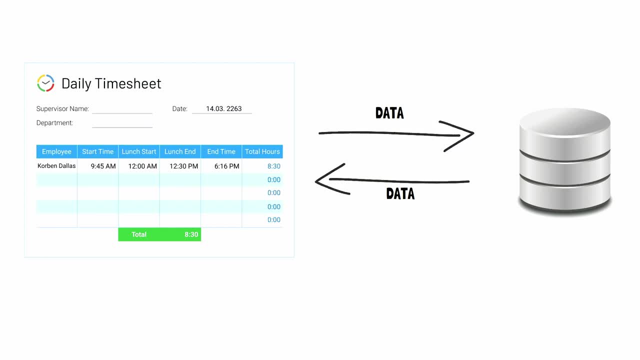 database is installed on your computer, the data is actually being stored into your computer memory. This is a simple example of how an application uses a small database to store, modify and retrieve data. When it comes to bigger applications or bigger companies, they need huge. 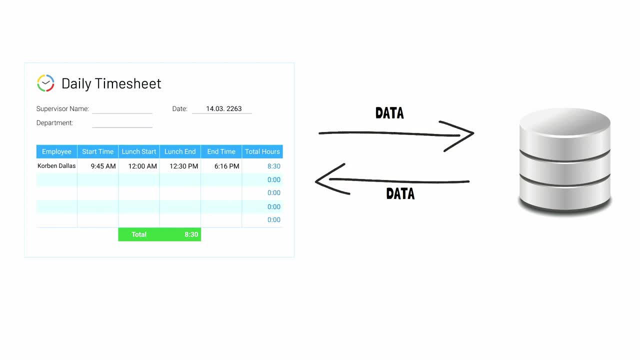 databases to store huge data which may be installed on large servers. This is true to any application that uses a database. The images, videos or posts or any other information that you see on Facebook is actually stored in a database And whenever you search for a specific post or friend Facebook, 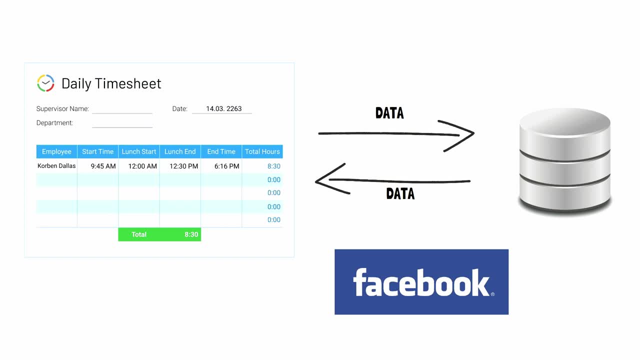 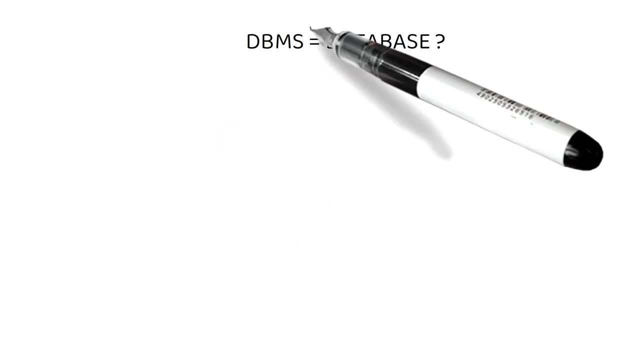 actually searches for this data in its database. So is database same as DBMS. But that's not entirely correct, because database is just a container that stores data, whereas DBMS, or database management system, is a software which is used to manage your database. You need DBMS to interact with the database: to store, modify, retrieve. 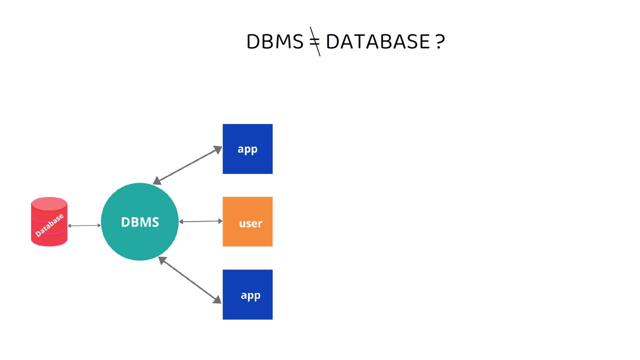 and protect data. DBMS is also required to create, modify and delete database. Users like you and me can use DBMS to enter commands in a specific language to interact with the database. Examples of DBMS can be MySQL, PostgreSQL, MongoDB, Neo4j, Cassandra, etc. 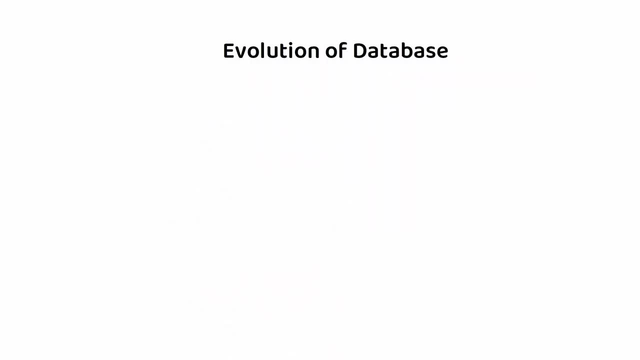 Evolution of database started in 1960s, when the first type of database were made, which was the flat file database. Here the data was stored in simple files such as CSV file or fixed length file, etc. Later on came the hierarchical database and then the network. 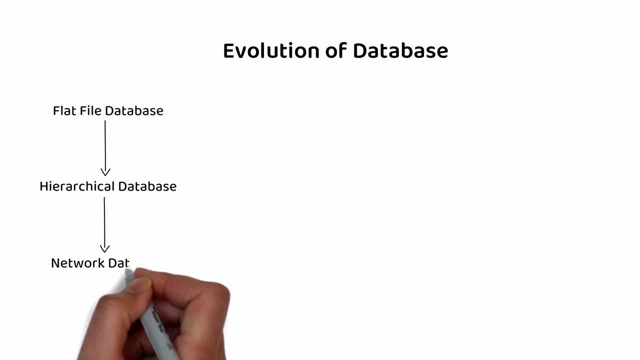 database. Both of these database stored data through parent-child relationship, But both of these database were incapable of storing complex data relationships, hence were soon replaced by relational database. Fast forward to 2020, in today's world, there are mainly two popular database types: relational- 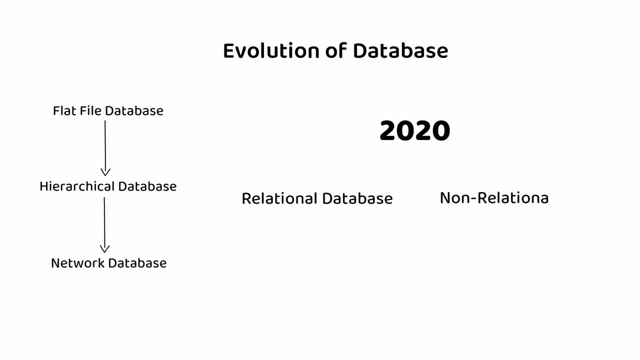 database and non-relational database. As per the usage, over 74% of the database used today are relational database, But due to the immense rise in data usage over the past decade, mainly due to social media platforms, non-relational database have become very popular. However, the biggest 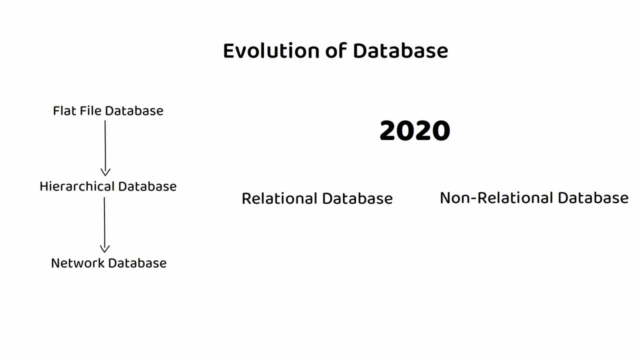 companies today, who store data related to millions of users every day, generally use combination of both relational and non-relational database, Hence both these database types are very popular and widely used. Oracle is the most widely used relational database, whereas MongoDB is the most widely used relational database. 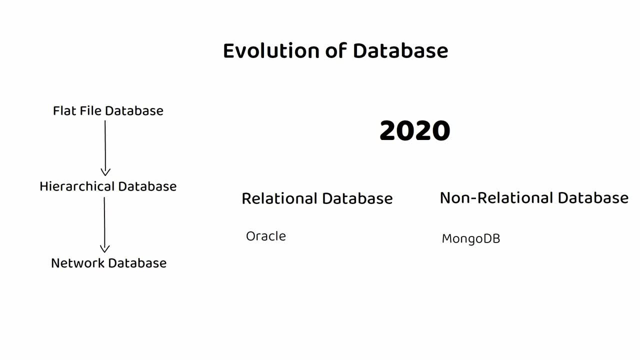 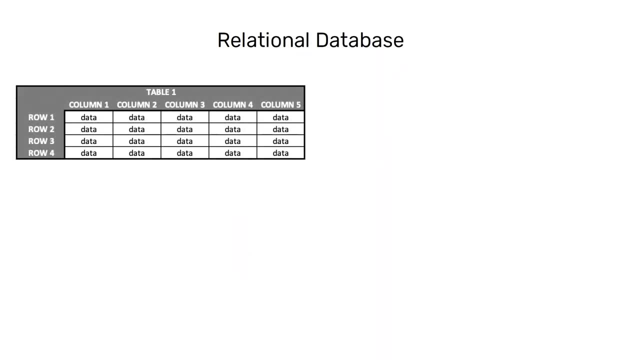 Oracle is the most widely used relational database, whereas MongoDB is the most widely used non-relational database. Let's briefly look at each of these database types. Relational Database: In a relational database, data is stored through collection of tables. These tables are related to one another. 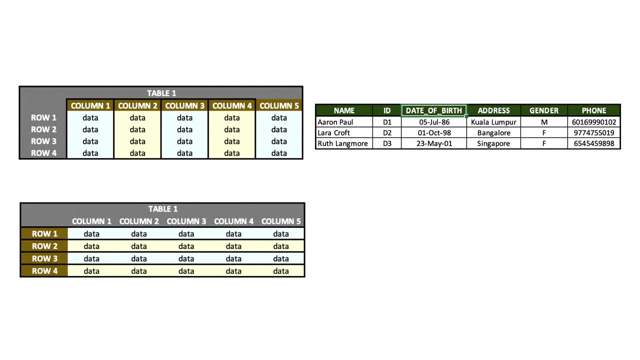 Each table consists of columns and rows. Each column has a name and a data type. Data type can be said as a data rule which is associated to every column. Only those data that satisfy this data rule can be inserted in the specific column. A row can be treated as a record, which is formed by single or multiple columns. 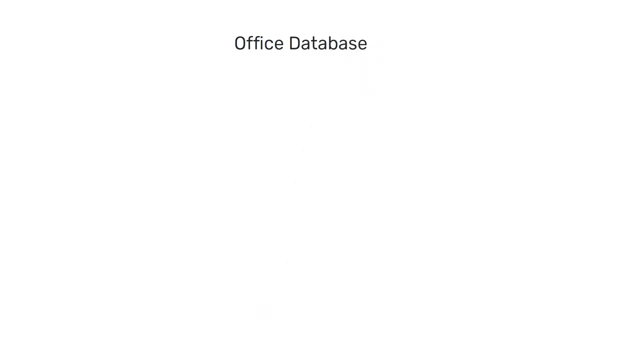 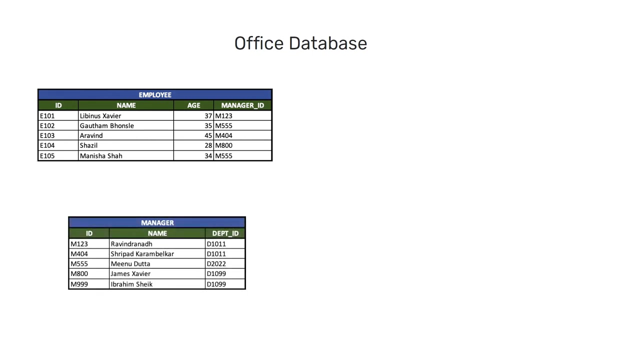 As an example, if we consider an office database, it will have information related to employees, managers and departments. These details are stored in different tables but these tables will be related to each other through certain columns. Here, employee and manager table is related through the manager ID column, which is present in the manager ID column. 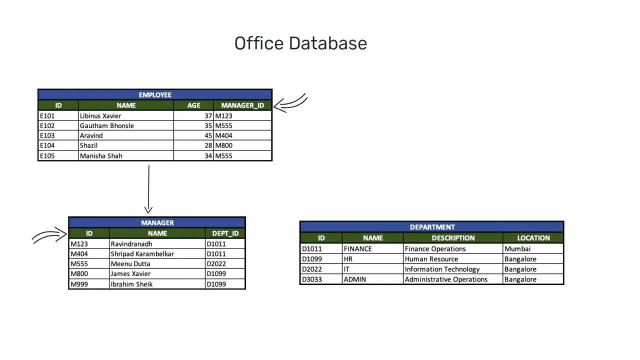 Here, employee and manager table is related through the manager ID column, which is present in both these tables. In a relational database, foreign key constraint is used to form relation between different tables. Similarly, manager and department tables are related through the department ID column. As you can see, employee and the department. 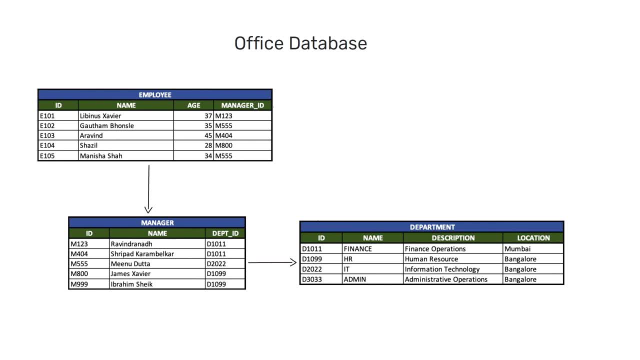 table are not directly related to each other, But still it is possible to fetch data from the employee table, based on specific conditions, from the department table. This is how relational database works. Information is scattered across multiple tables which are related to one another. Hence, using table relations, it is possible to retrieve. 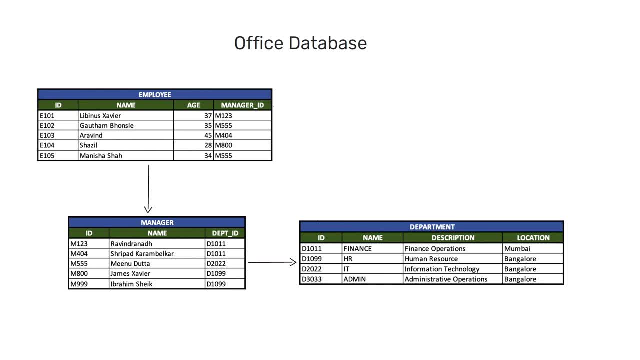 data from different tables In a relational database. using DBMS, you can enter commands in specific language to store, retrieve and modify data. This specific language is SQL or Structured Query Language. SQL is a programming language which follows a standard format for querying data across different relational databases. Most of the financial 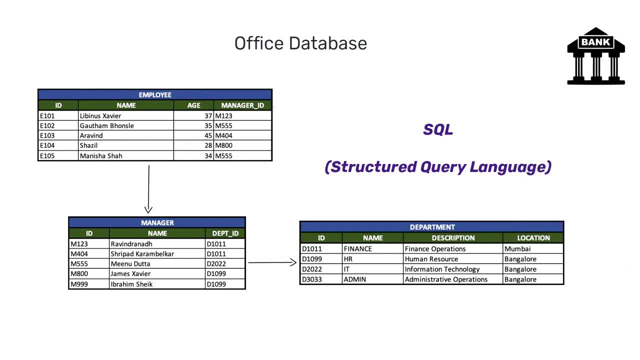 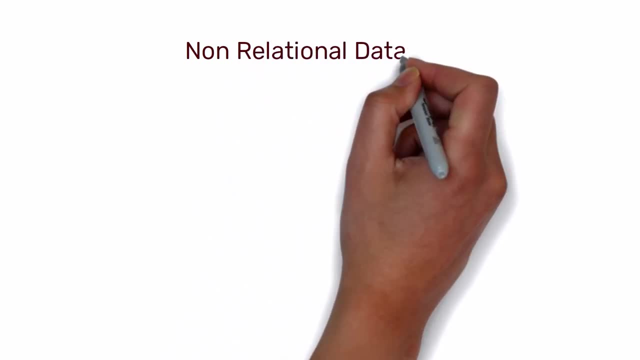 institutions, such as the financial institutions, are using this format. Most of the financial institutions, such as bank or insurance companies, use relational database. Examples of relational database are Oracle, MySQL, Microsoft SQL Server, PostgreSQL, etc. Non-Relational Database. When it comes to a non-relational database, 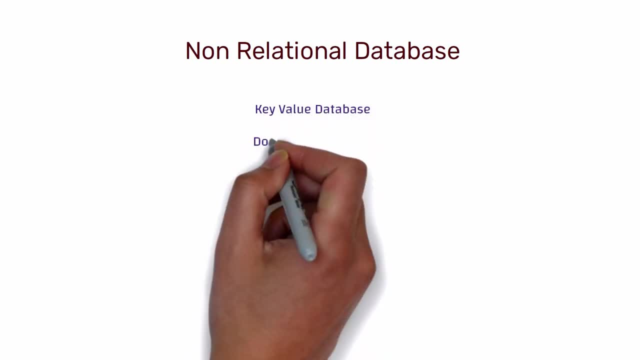 there are several categories of database, such as Key Value Store, Document Database, Graph Database, Wide Column Database, Search Engine Database, Time Series Database, etc. Each of these databases store data differently and are useful for managing specific types of data. Let's briefly look at a few of them: Key Value Database. 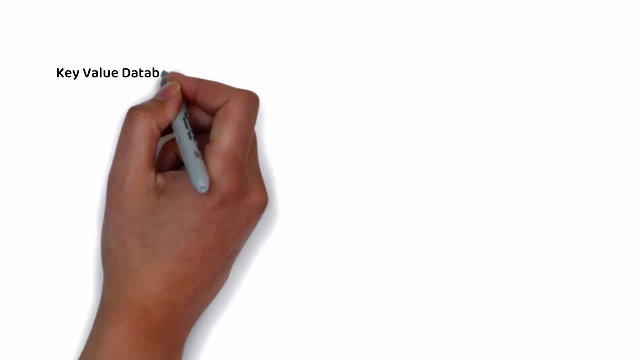 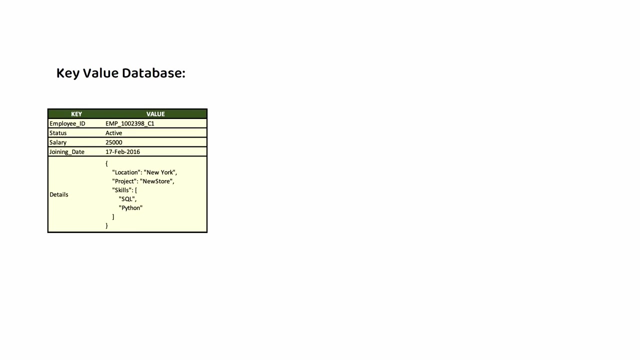 Also called as Key Value Store. It is the simplest of the non-relational database and, as the name suggests, every data stored in this database will be assigned to a key To store data. you provide a key and a blob of data, such as an image, text file, JSON object. 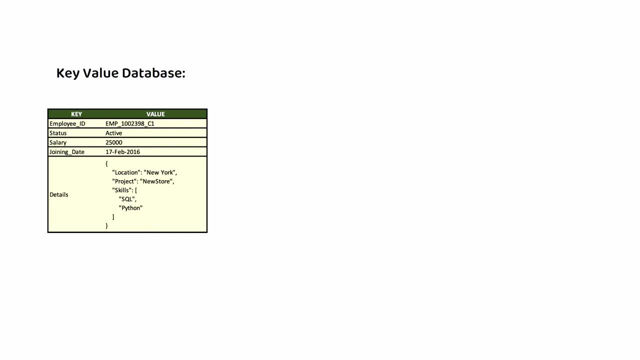 etc. Once saved, to retrieve the data, just provide the key. Key Value Database are very useful to store certain types of data, such as configuration data, state information or any data that might be represented by a dictionary or a hash in a programming language. Examples can be Redis: 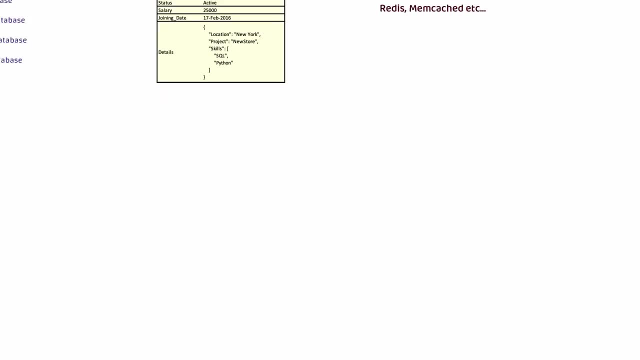 Database, Memcached Database, etc. Document Database, Also called as Document Store- These are these also use Univision database. They are unique key to identify data stored in database. However, unlike Key Value Store, Document Database stores data in structured format called documents, often using JSON, Vsun or XML format. 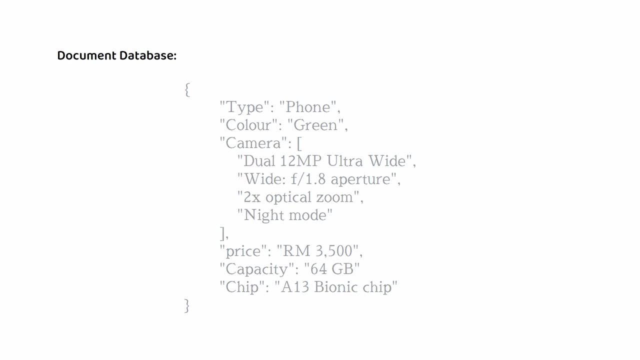 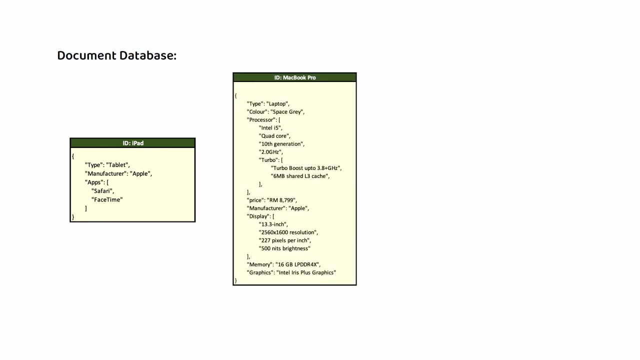 Though each document within this database has structured data, there is no specific format to be followed for all documents. Each document can have its own structure which the database understands. So, unlike Key Value Store, the data stored in Document Database can be queried and analyzed. Examples can be MongoDB, CouchDB, etc. 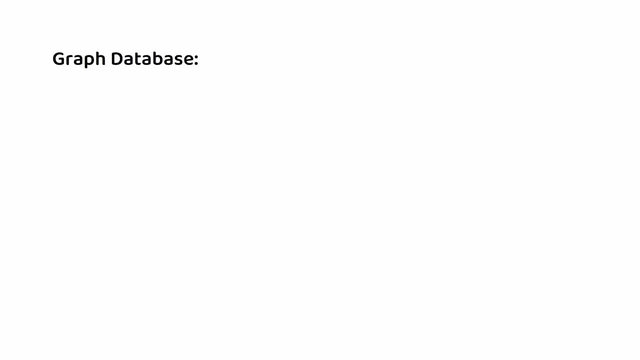 Graph Database. Graph Database falls under the bracket of Non-Relational Database and follows a different approach to forming relationships between data. Rather than using tables and foreign keys to form relation, Graph Database forms relation by using nodes, edges and properties. Data is represented through individual nodes and each node can have multiple properties.